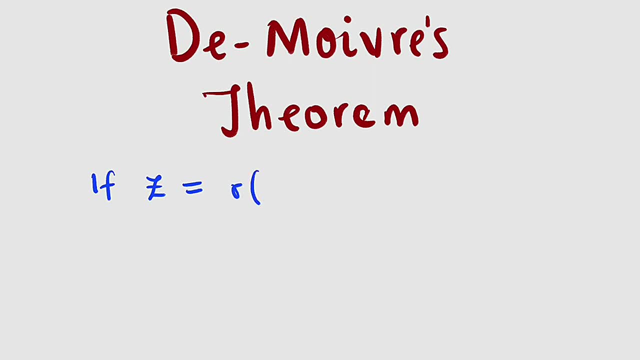 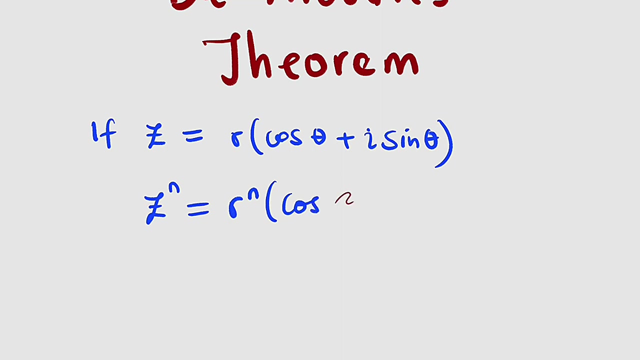 which is written in a polar form: r multiplied by cosine of theta plus i sine of theta. it stated that z to the power of n, for which n is an integer. this is the same thing as r raised to the power of this n, then multiplied by cosine of this n, multiplied by the angle, then plus i sine. 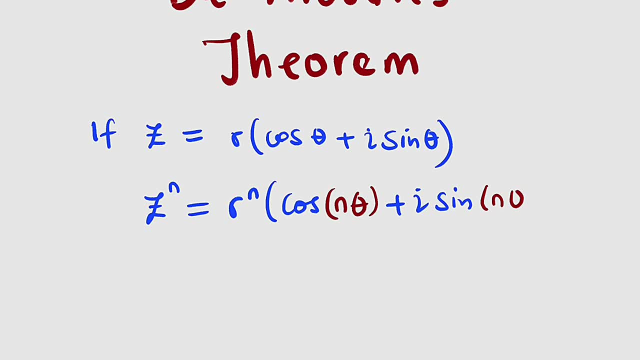 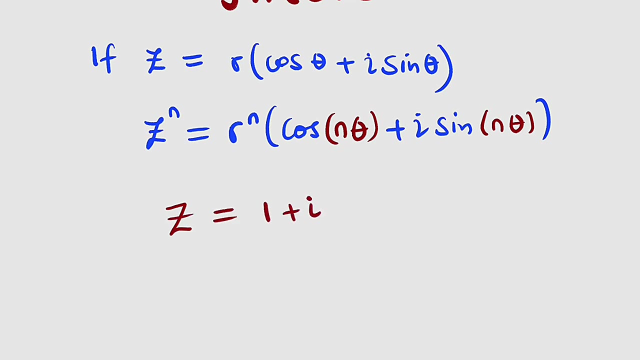 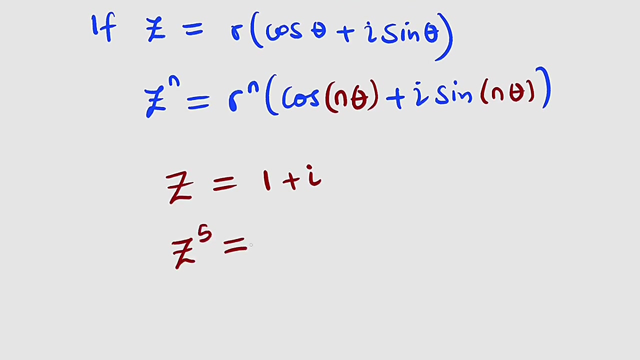 of that same n multiplied by the angle. So this is exactly what the Moeber theorem stated. So let's give an example to see how it works. for example, let a complex number, z be equal to one plus i, very simple, complex number. so what if we want to raise z to the power of five? you know, it is the same thing as one plus i to the. 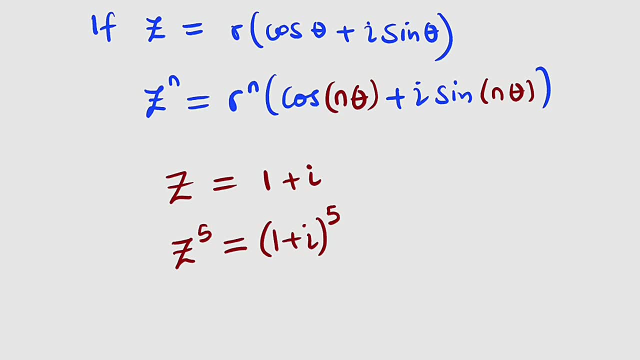 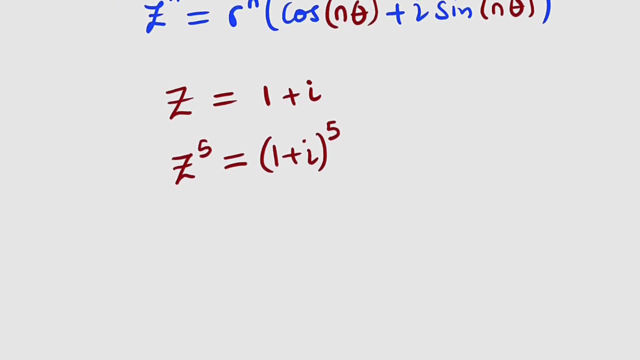 power of five, which means one plus i times one plus i times one plus i after five places, which is a very big work, right? so instead we can apply this formula in evaluating this: all we need is r and theta, so let's find r. so from here, if we are looking for, 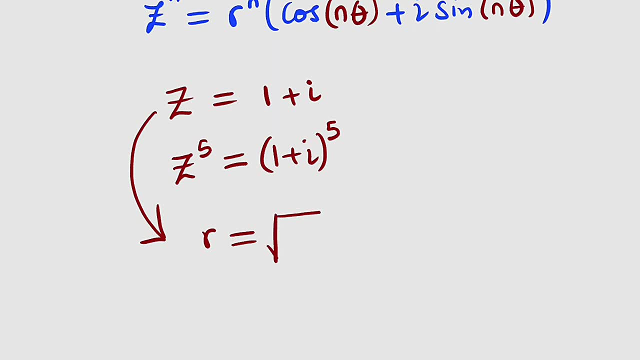 the r, which is the modulus. it is equal to the square root of a plus b. a is the real part and b is the imaginary part. a is one squared plus b, which is just the coefficient of. i is also one squared. one squared and one squared are all one. one plus one is equal to two. therefore, r is 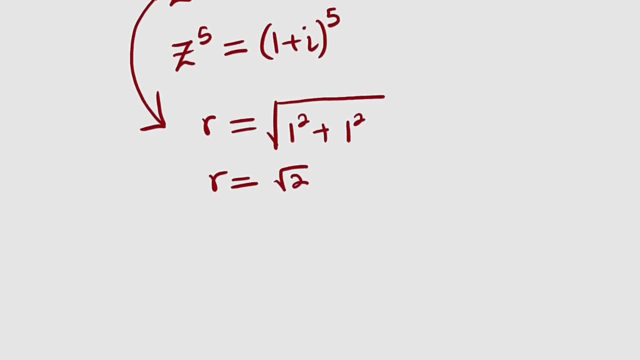 equal to square root of 2.. Now for the angle theta. you know it is the same thing as tan inverse of what: b divided by a. b is 1, a is 1.. 1 divided by 1 is equal to 1. 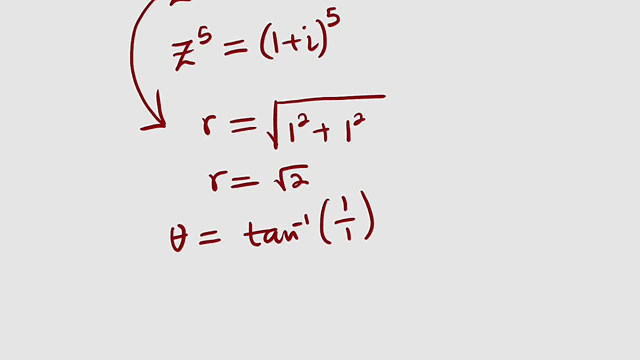 and tan inverse of 1 is 45 degrees, or pi by 4.. So let's use the radian theta equal to pi by 4.. Therefore the complex number in the polar form is now equal to r, which we have as square root of 2, multiplied by cosine of this angle. pi by 4, then, plus i multiplied. 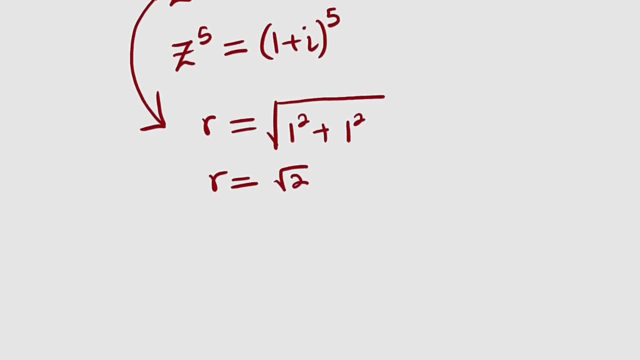 equal to square root of 2.. Now for the angle theta. you know it is the same thing as tan inverse of what: b divided by a. b is 1, a is 1.. 1 divided by 1 is equal to 1. 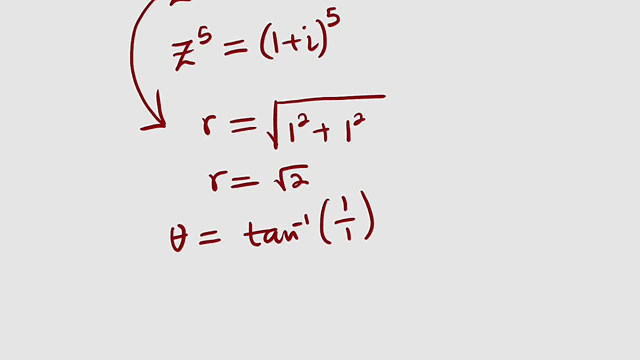 and tan inverse of 1 is 45 degrees, or pi by 4.. So let's use the radian theta equal to pi by 4.. Therefore the complex number in the polar form is now equal to r, which we have as square root of 2, multiplied by cosine of this angle. pi by 4, then, plus i multiplied. 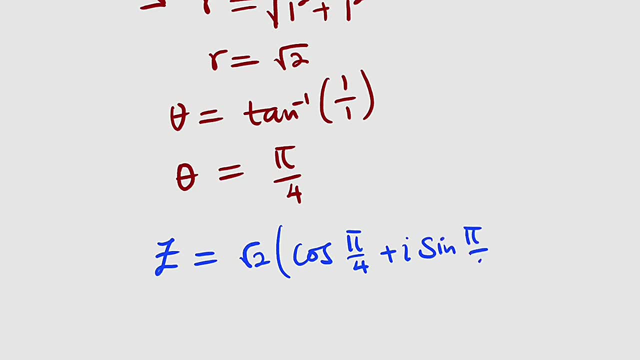 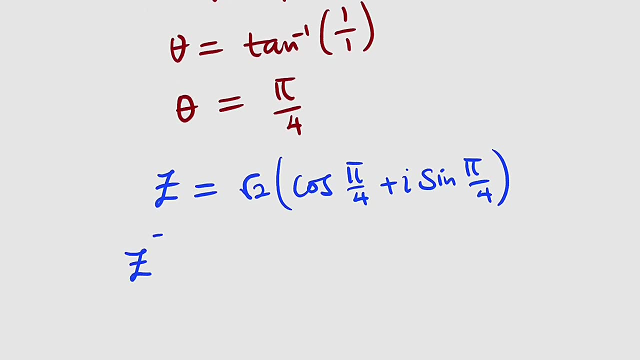 by sine of that angle, pi by 4.. But remember, we want to expand z to the power of 5.. So z to the power of 5, according to the Merber's theorem, it stated that it is the same thing as r to that power, then multiplied by cosine of what That n multiplied. 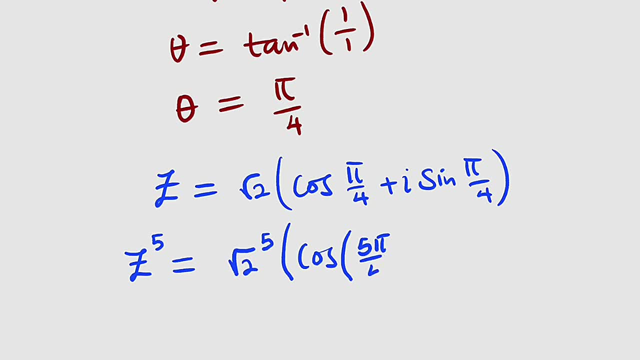 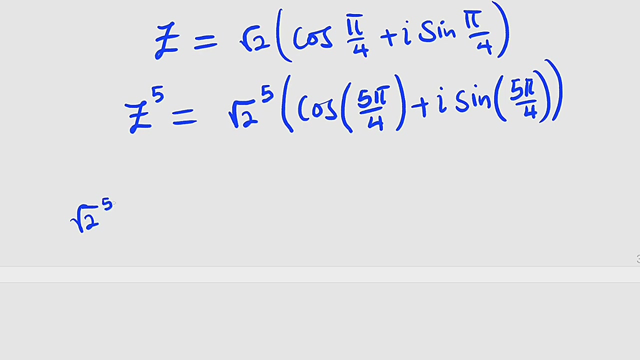 by the angle that is 5 pi by 4, then plus i sine of that same 5 pi by 4.. So now let us simplify this. What is root 2 to the power of 5? power of 5. let me do it here: root 2 to the power of 5 is equal to root of 2 to. 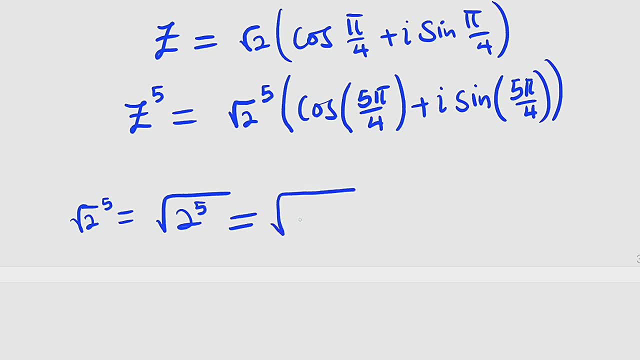 the power of 5 and this is equal to root of what. 2 to the power of 1, multiplied by 2 to the power of 4, according to law of indices, and 2 to the power. 4 is 16. square root of 16 is 4, so this is the same thing as 4, root of what 2. 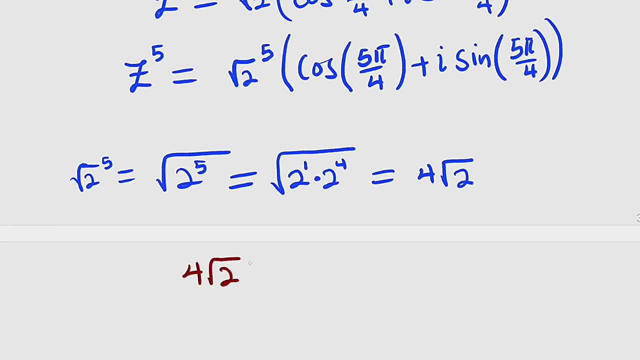 therefore we have: 4. root of 2 multiplied by cosine of 5 pi by 4 is equal to negative root 2 divided by 2. negative root 2 divided by 2, then plus I, multiplied by sine of 5 pi by 4, is the same thing. negative root 2 divided by 2. 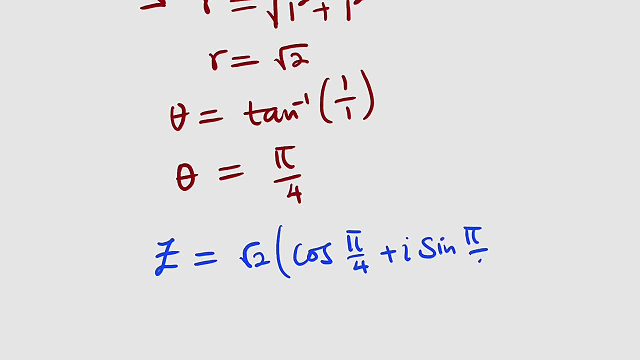 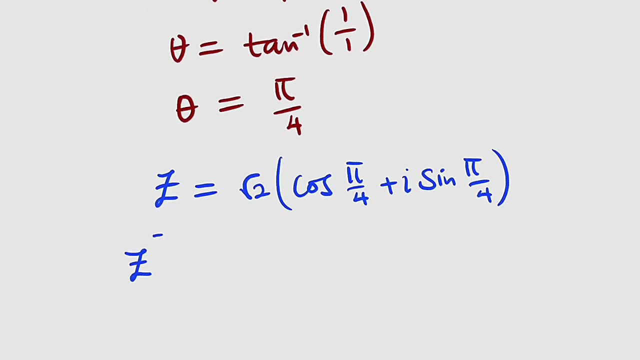 by sine of that angle, pi by 4.. But remember, we want to expand z to the power of 5.. So z to the power of 5, according to the Merber's theorem, it stated that it is the same thing as r to that power, then multiplied by cosine of what That n multiplied. 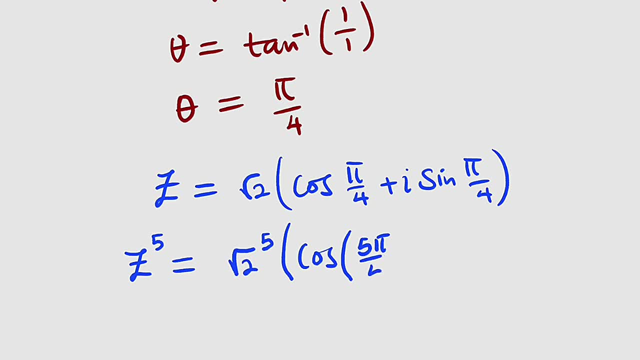 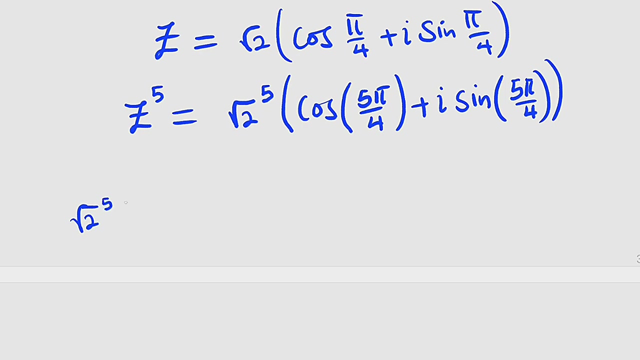 by the angle that is 5 pi by 4, then plus i sine of that same 5 pi by 4.. So now let us simplify this. What is root 2? power of 5? let me do it here: root 2 to the power of 5 is equal to root of 2 to. 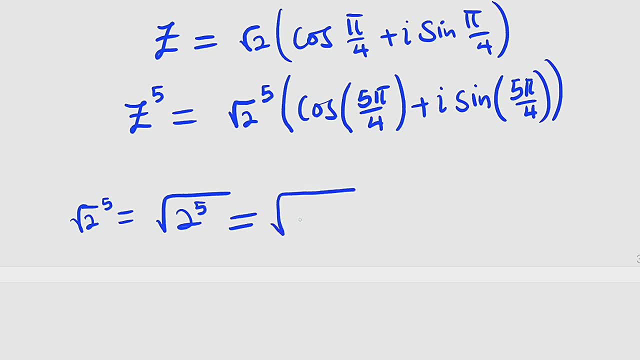 the power of 5 and this is equal to root of what. 2 to the power of 1, multiplied by 2 to the power of 4, according to law of indices, and 2 to the power. 4 is 16. square root of 16 is 4, so this is the same thing as 4, root of what 2. 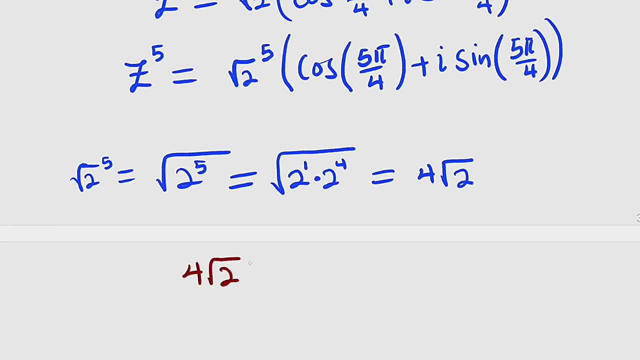 therefore we have: 4. root of 2 multiplied by cosine of 5 pi by 4 is equal to negative root 2 divided by 2. negative root 2 divided by 2, then plus I, multiplied by sine of 5 pi by 4, is the same thing. negative root 2 divided by 2. 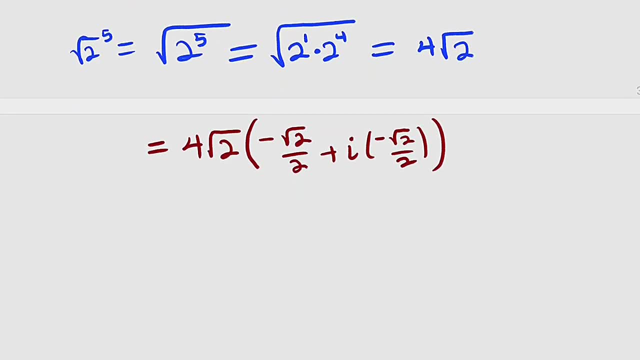 so what we are going to do next is to expand because of this negative multiply by a positive number. we have negative: 4 root 2 multiplied by root 2 divided by 2, then plus this is also negative, we have negative of what 4 root 2 multiplied by root 2 divided by 2 root 2 times root 2 is what 2 2 times 4 is. 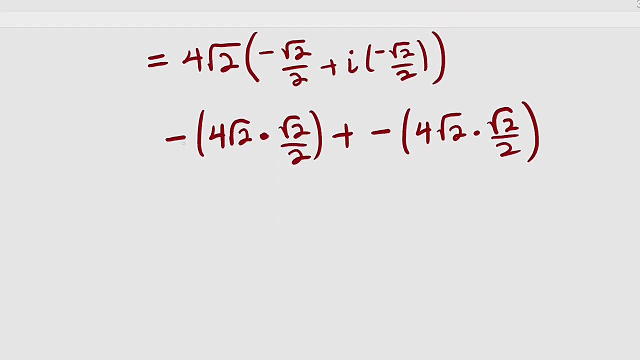 8. 8 divided by 2 is 4.. But because of this negative, we have negative 4.. This is negative, 4.. This and this will become negative. This is negative And this is also 4.. But remember, we have our i here. 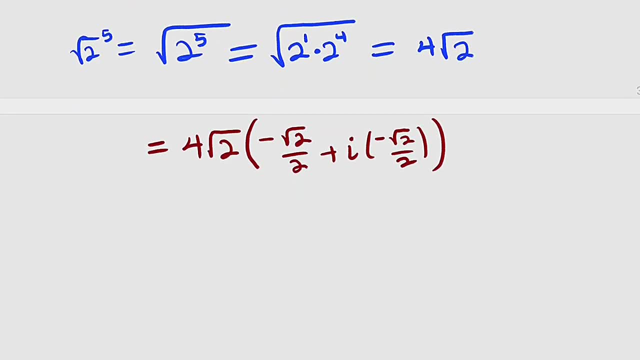 so what we're going to do next is to expand because of this. we're going to expand this negative multiplied by a positive number, we have negative 4 root 2 multiplied by root 2. divided by 2, then plus, this is also negative. we have: 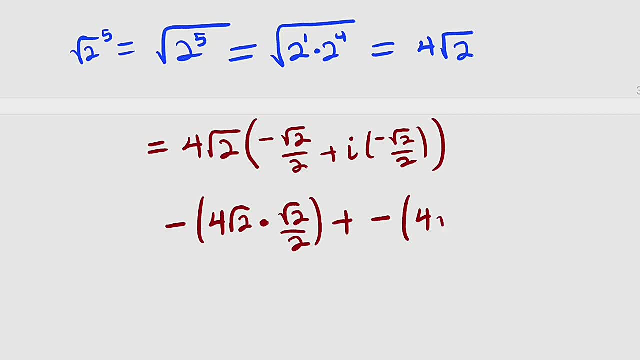 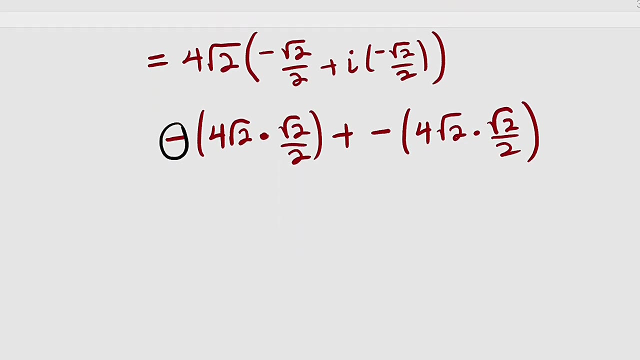 negative of what 4 roots to multiply by root 2, divided by 2 root, 2 times root 2 is what 2, 2 times 4 is 8. 8 divided by 2 is 4. but because of this negative we have negative 4. this is negative 4. 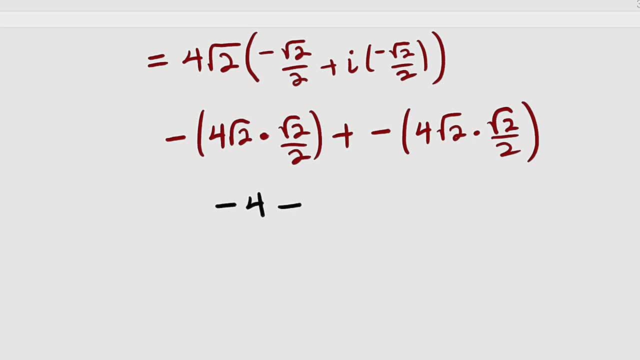 this and this will become negative. this is negative and this is also 4, but remember, we have our I here, so we have 4 I, which implies that 1 plus I, raised to the power of 5, is the same thing as negative 4 minus 4 I, according to the. 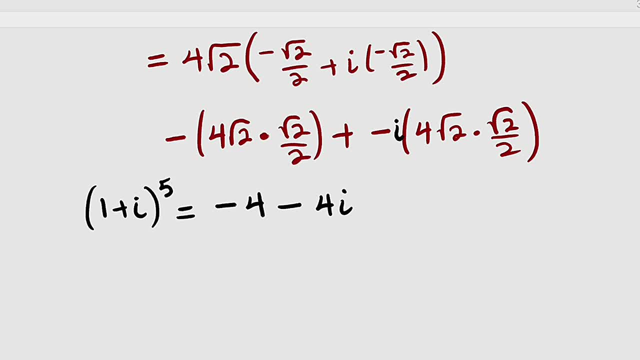 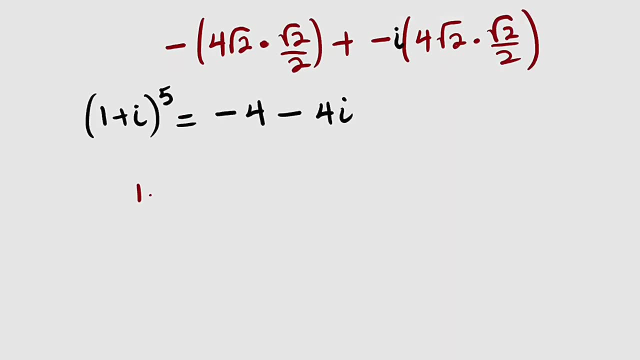 Moevers theory. but now I want us to use our normal expansion to expand this to see whether we're going to get negative 4, negative 4 I. so 1 plus I raised to the power of 5, which is the same thing as 1 plus I multiplied by 1 plus I multiplied by 1. 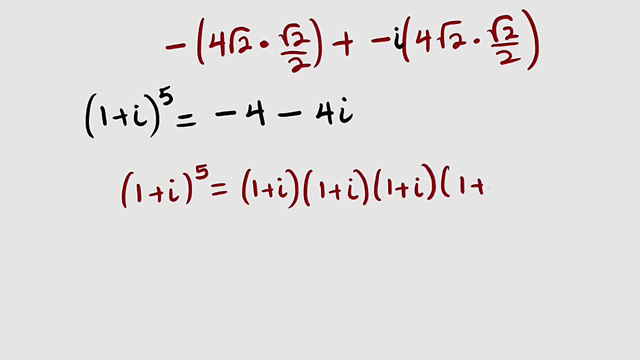 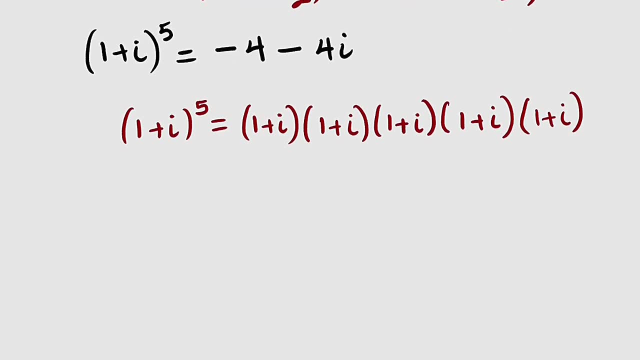 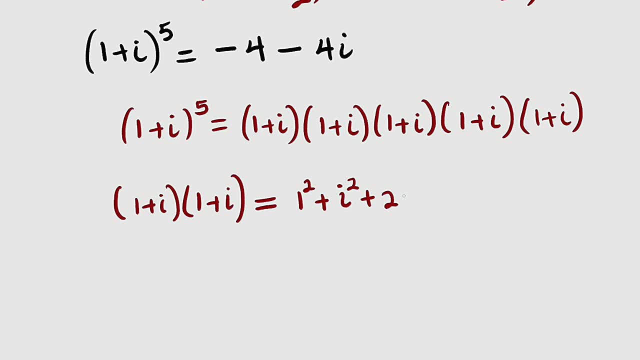 2, multiplied by first time, multiplied by second time, 1 times. I is just I right. this is equal to 1 Square. this one male, very important. yes, that's why this is equal to 4 times 6 plus 3 times 1000 square. 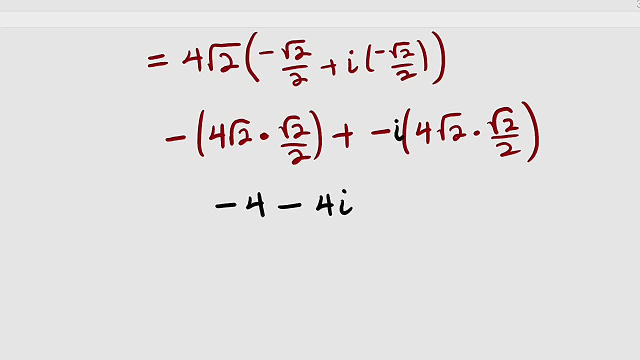 So we have 4i, which implies that 1 plus i, raised to the power of 5, is the same thing as negative 4 minus 4i, according to De Moivre's theory. But now I want us to use our normal expansion to expand this. 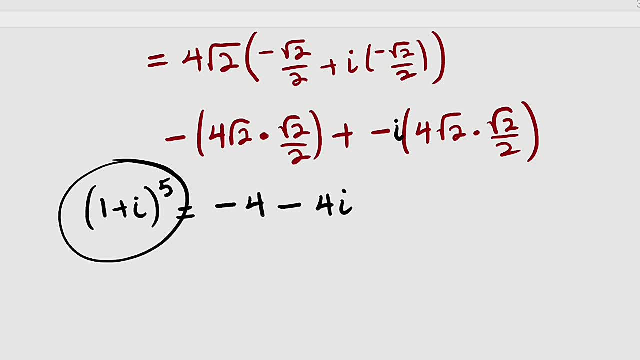 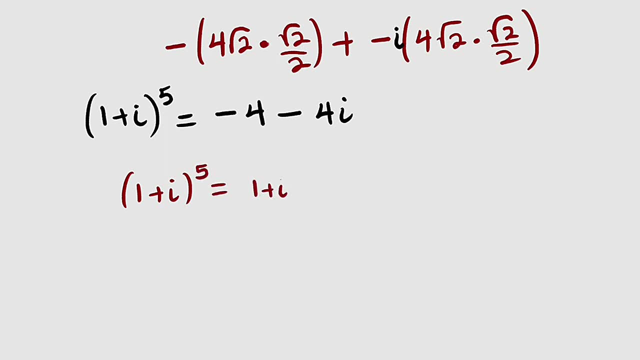 to see whether we're going to get negative 4, negative 4i. So 1 plus i raised to the power of 5, which is the same thing as 1 plus i multiplied by 1 plus i multiplied by 1 plus i. 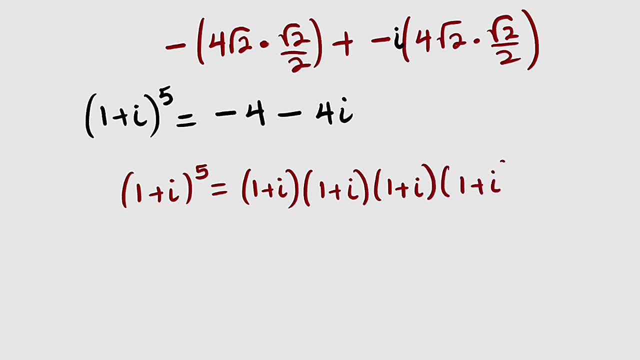 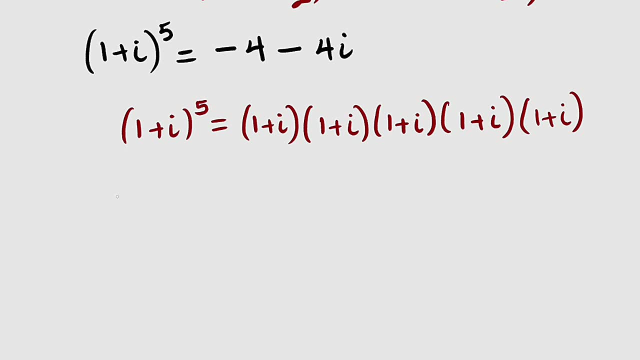 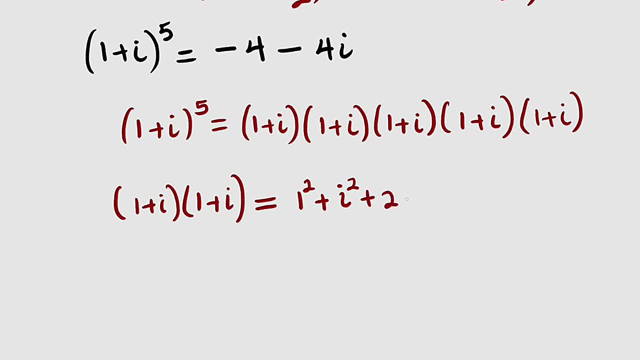 plus 2, multiplied by first time, multiplied by second time, 1 times. i is just. i right. This is equal to 1, squared is 1, but i squared is negative 1, according to definition, then plus 2i. 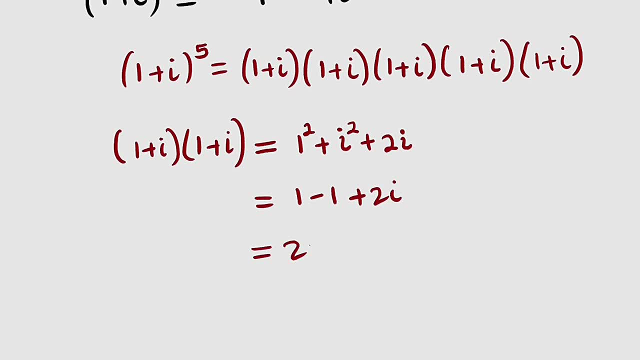 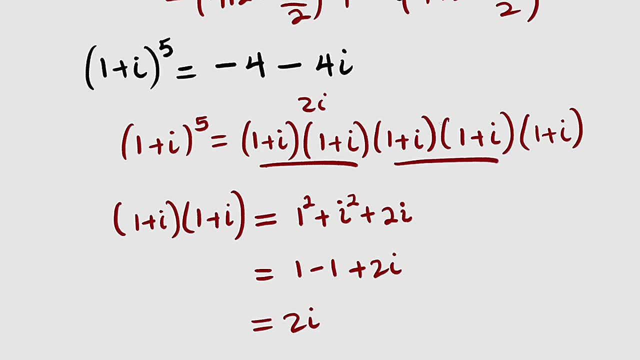 1 minus 1 is 0, so we have only 2i. So we have seen that the first 2 is equal to 2i. The second 2 will also be equal to 2i. So what if we should multiply first 4 together? 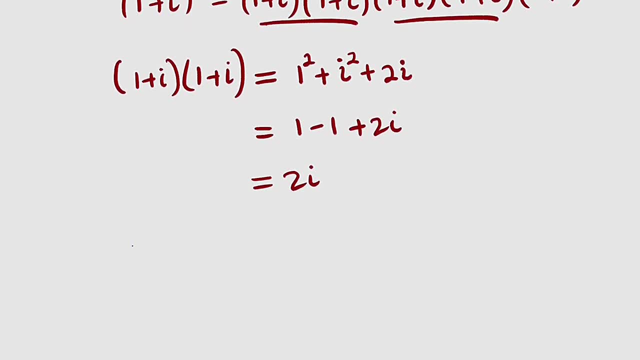 leaving 1 extra left- 1 plus i, multiplied by 1 plus i multiplied by 1 plus i multiplied by 1 plus i, We have seen that the first 2 will give us 2i and the second 2 will also be equal to 2i. 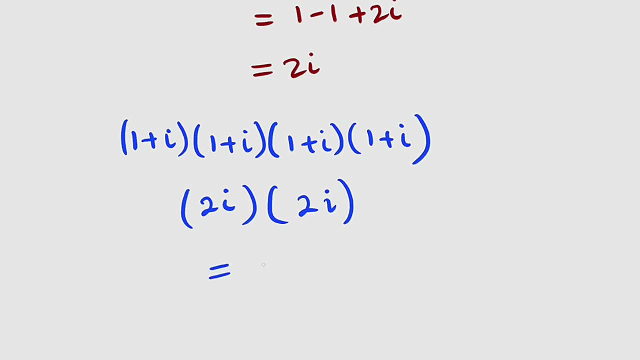 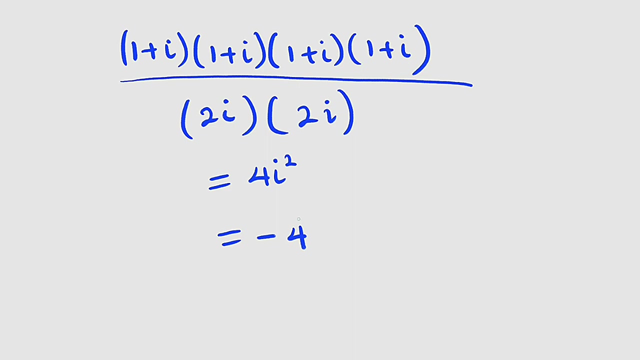 We have 2i times 2i, which is going to give us 4i squared. But remember that i squared is equal to what Negative 1, therefore, the whole of this will be negative 4.. Now, the expression of all of this: 4 is equal to negative 4.. 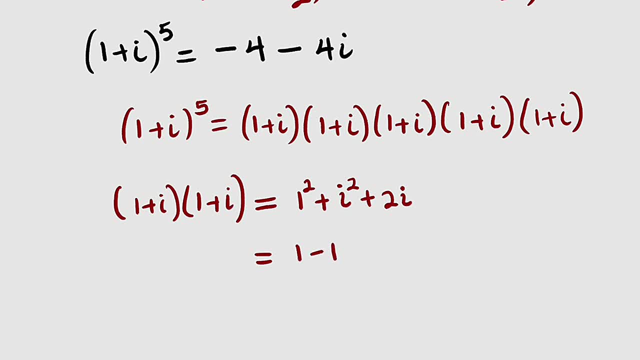 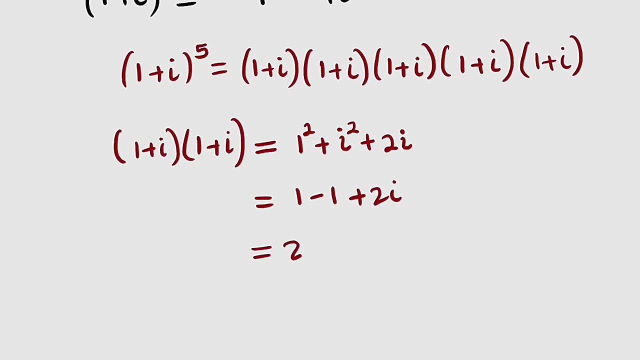 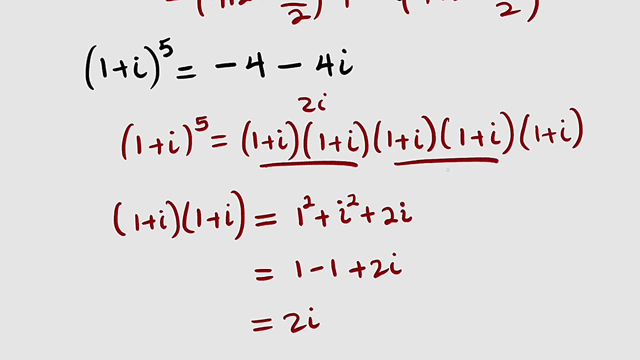 again, this equals to 12.. 1- but i squared- is negative 1 according to definition. then plus 2i, 1 minus 1 is 0, so we have only 2i. So we have seen that the first two is equal to 2i. The second two will also be equal. 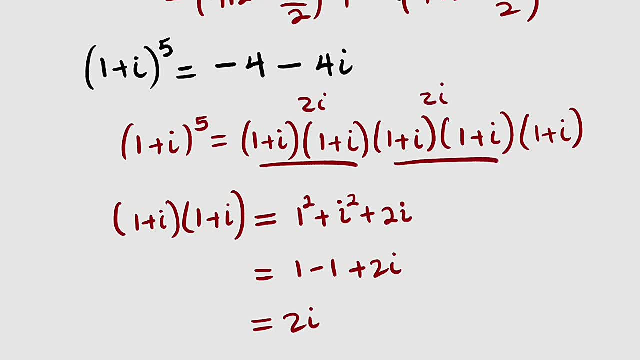 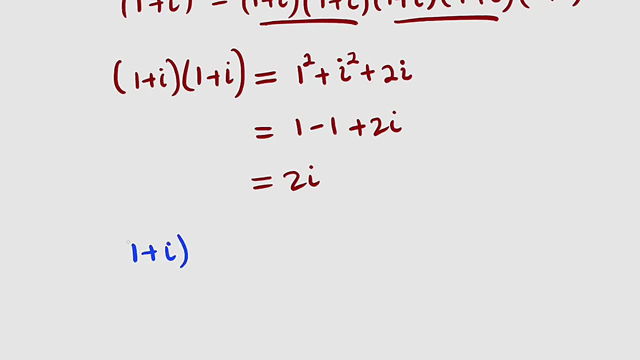 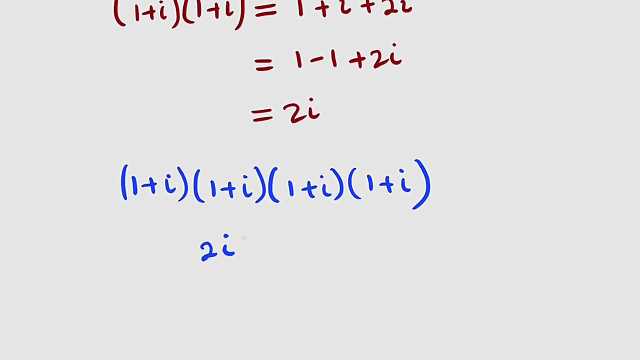 to 2i. So what if we should multiply first four together, leaving one extra left, 1 plus i, multiplied by 1 plus i multiplied by 1 plus i multiplied by 1 plus i? We have seen that the first two will give us 2i and the second two will also be equal to 2i. We have 2i times 2i. 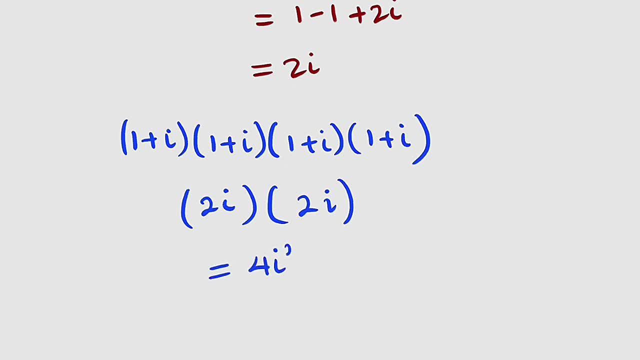 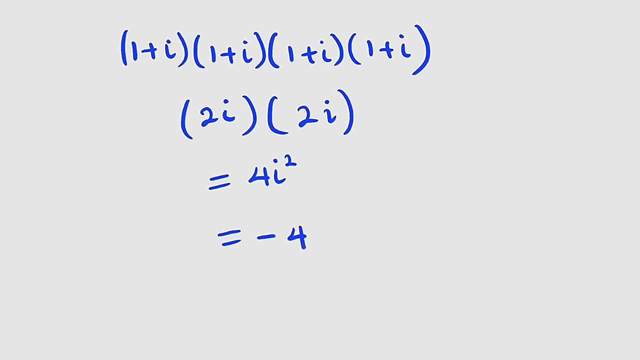 2i squared, So we have 2i squared, So we have 2i squared. Therefore, the whole of this will be negative 4.. Now, the expression of all of this: 4 is equal to negative 4.. But remember, we have: 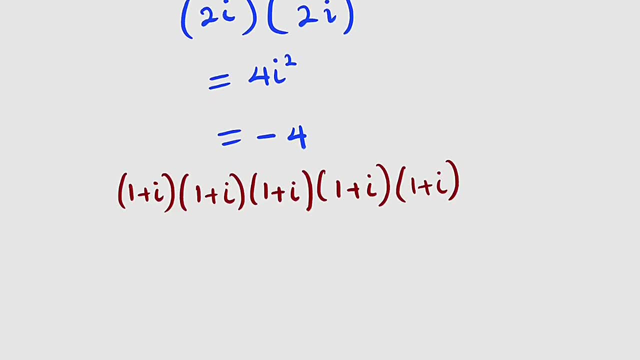 one left, which is what 1 plus i. So, since the first 4 is just negative 4, all we have to do is to take this negative 4 and multiply it by 1 plus i. By doing so, negative 4 times 1 is negative 4. 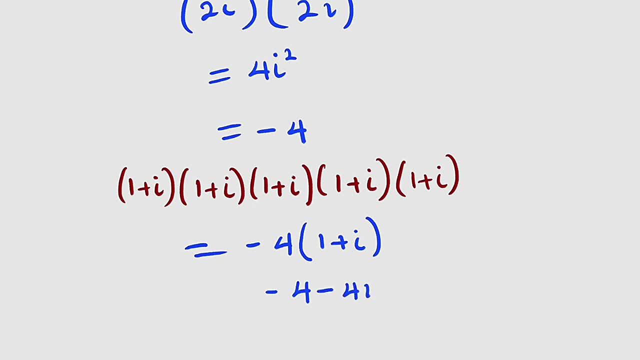 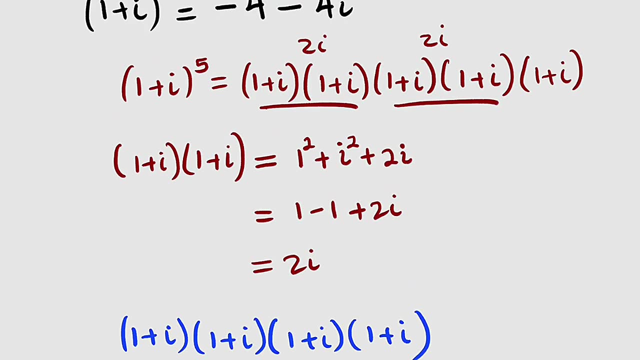 and negative 4 times, i is negative 4.. So we have 2i squared i, which implies that z to the power of 5 is equal to negative 4, negative 4i, which is exactly the same thing as using the Moeber's theorem to expand that z to the power of. 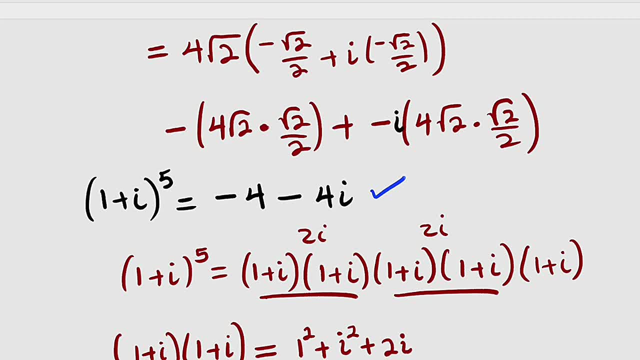 5. So, since we have seen that it is applicable subsequently, we're not going to be using this normal expression. We'll be applying the Moeber's theorem to expand our complex numbers. And this is all I have for you today. Thank you for watching. Do share to your learning colleagues. 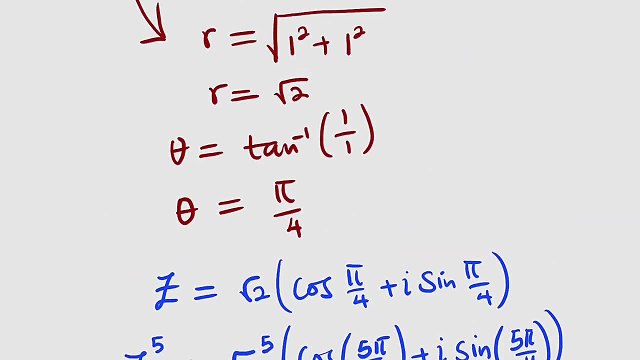 And don't forget to subscribe to my YouTube channel for more exciting videos. Bye, bye.